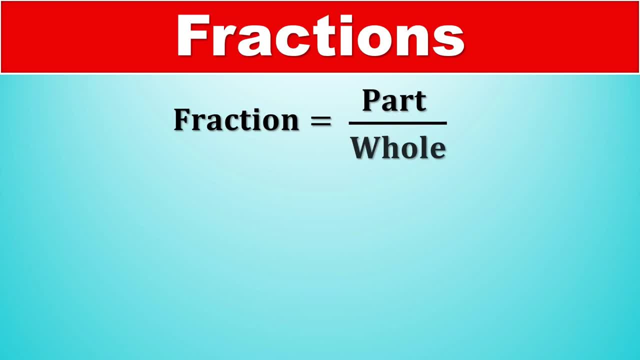 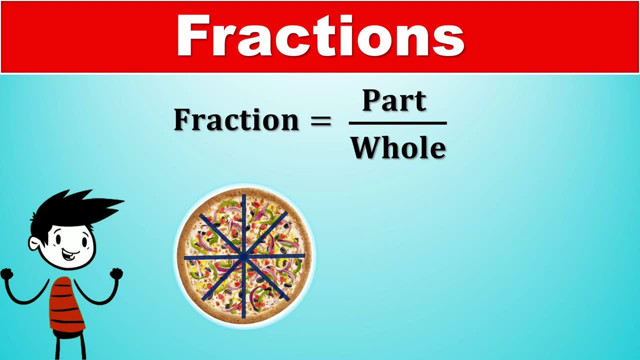 Now, again, we'll take an example of a pizza for this, and this time we're gonna split it into eight slices, and so that an amount of pizza will be zero neurotransmitters. so we'll simply divide. denominator of this fraction will be 8, as there are 8 total slices. Now let's begin. 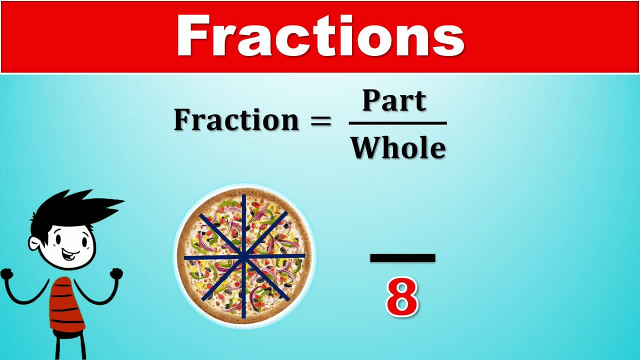 taking slices from this pizza And we'll count up as we go. So, starting with 1: eighth of the pizza, 2 eighths of the pizza, 3 eighths of the pizza, 4 eighths of the pizza, 5 eighths, 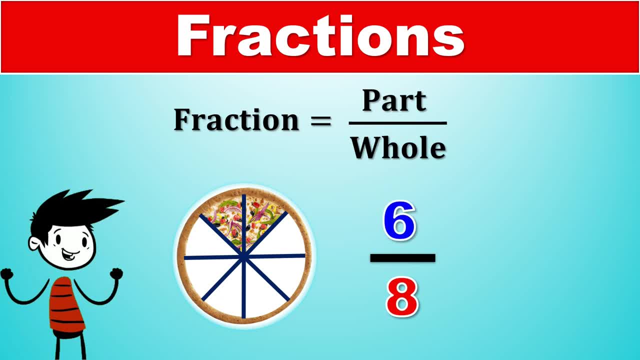 of the pizza, 6 eighths of the pizza, 7 eighths of the pizza and finally, 8 eighths of the pizza, Which is actually just 1, because any number divided by itself always equals 1.. 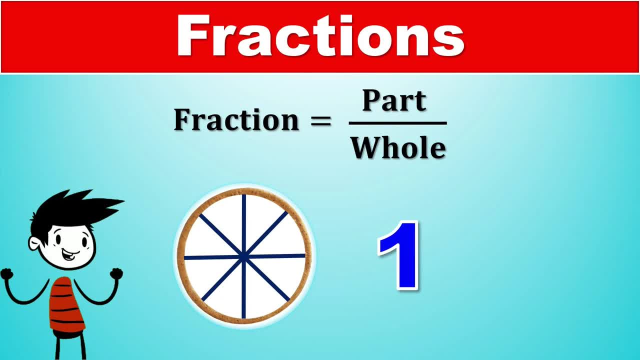 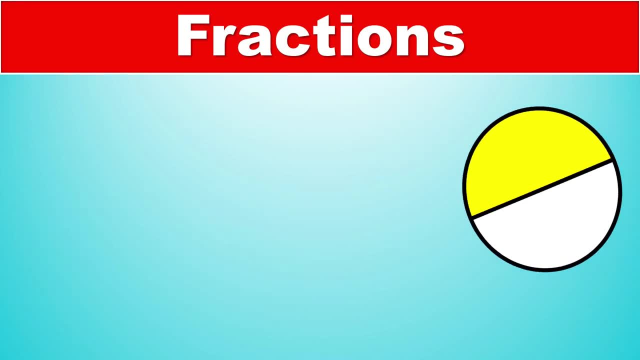 Now let's take a look at what these top and bottom numbers mean in detail. So here we have another circle And this time, as you can see, we've split it into two parts. So here we have another circle And this time, as you can see, we've split it into two parts. 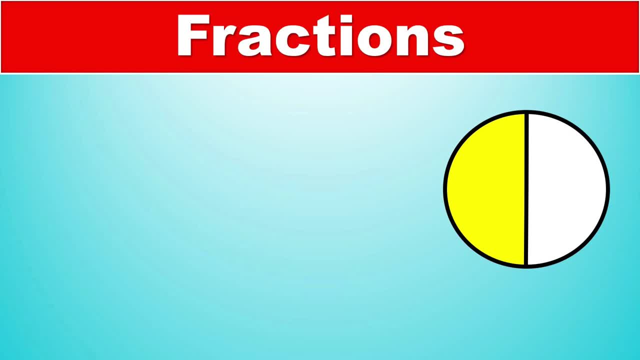 So here we have another circle, And this time, as you can see, we've split it into two parts. So let's take a look Now. the fraction that represents the shaded part of this circle is 1 half, which you can write as 1 over 2, or 1 by 2.. Now the top number here, 1, is. 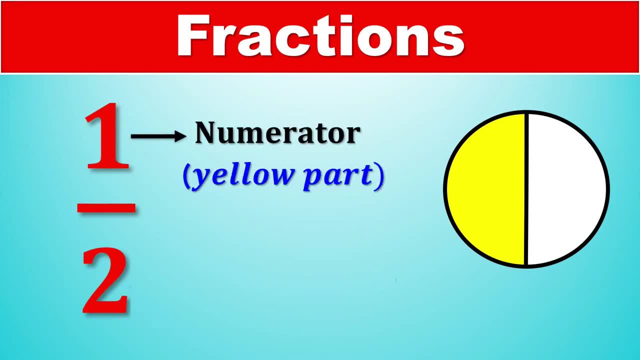 called the numerator, And it is the yellow part, It's the shaded part in our circle, And the bottom number, the 2, is the denominator. The denominator the total number of parts in our circle, And so the total fraction. 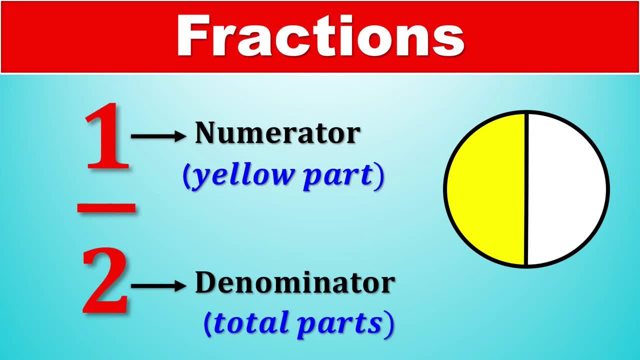 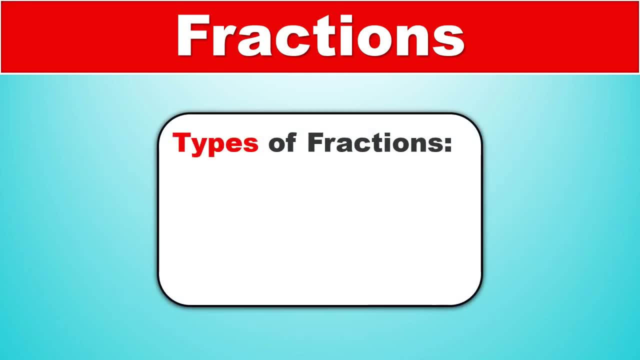 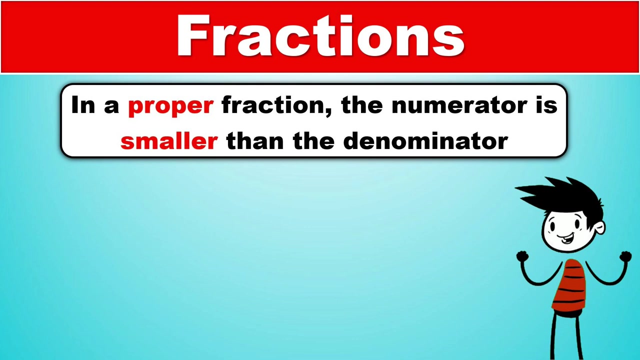 of the yellow parts of our circle is 1 half. Now let's go to types of fractions. There are three major types: Proper fractions, improper fractions and mixed fractions. In a proper fraction, the numerator- the top number- is smaller than the denominator- the bottom number.